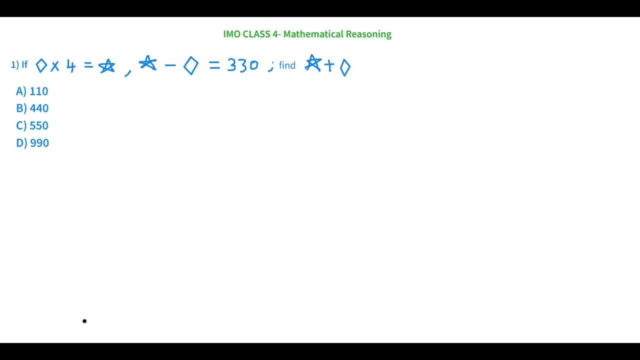 So in this video we are going to learn IMO class 4.. This is International Math Olympiad, class 4, Mathematical Reasoning Skill. I have already made a video about all the topics of IMO class 4.. You can refer that. The link is given below in the description, or you can. 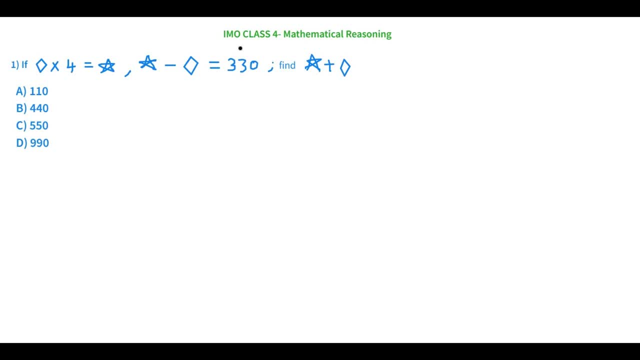 simply click on the I button given above. So this topic of IMO, class 4, Mathematical Reasoning Skill, was requested from a subscriber, So I am making this video. So let's see the first question for today. If diamond times 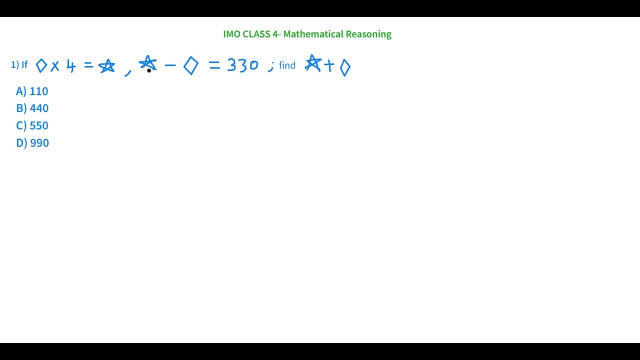 4, that is 4 times diamond equals star and star minus diamond equals 330, find star plus diamond. So we don't know the value of a star, we don't know the value of a diamond. So we have got two equations with us. That is 4 times diamond is a star and star minus. 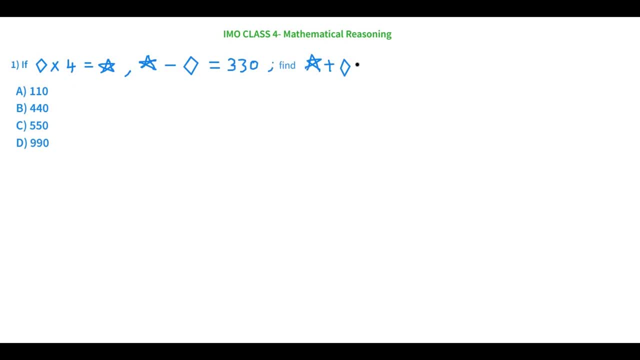 diamond is 330.. So we have to find the value of star. So let's find the value of a star and diamond. So we have two equations with us. So let's take the second equation, which is star minus a diamond equals 330.. So we have this equation. 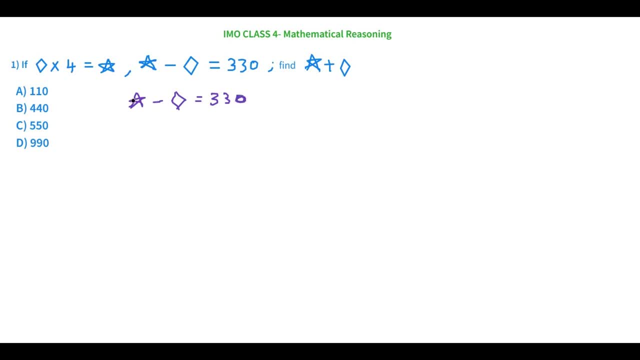 But we know what is a star. A star is nothing but 4 times of diamond. So in place of star I will put it as 4 diamond. So here I have: 4 diamond minus a diamond equals 330.. Right, So 4 diamond minus 1 diamond, we will get it as 3 diamond. So 3 diamond equals. 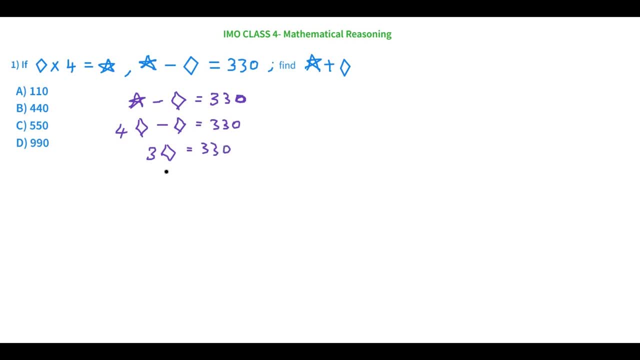 330.. So the value of 3 diamond is 330.. So what is the value of 1 diamond? 1 diamond equals 110.. So we know the value of diamond now. So now let's substitute this in the: 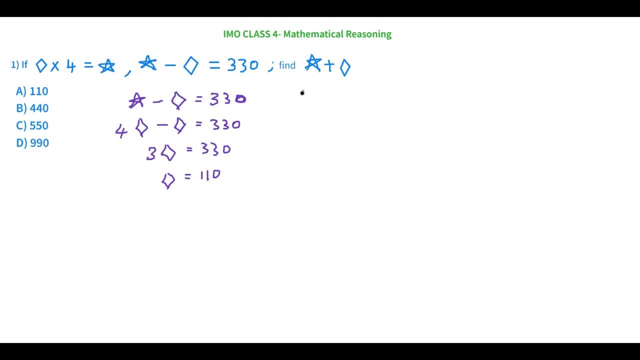 first equation, That is, diamond, is 110.. So 4 times 110 equals a star Right. So star equals 440.. So now we know the value of a diamond, We know the value of a star, So 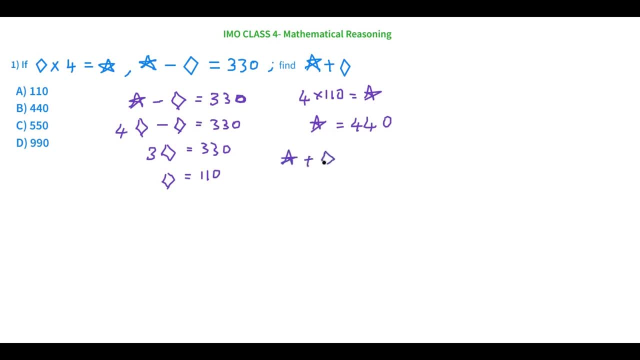 what is to be found? Star plus diamond, So what is star plus diamond? Star's value is 440 plus 110, which is 550.. So we have got our answer: 550.. Star plus diamond, So that is 440 plus 110, which is 550.. So our answer is 550. 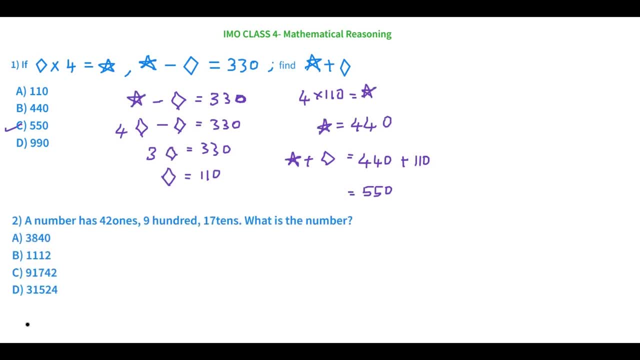 Isn't it easy. Now let us see the second question for today, which is a number has 42 ones, 917 tens. What is the number? We have our 4 options here. Option A is 3840.. Option B is 1112.. Option C is 91742.. Option D is 31440.. Option C is 91742.. Option D is 31440.. 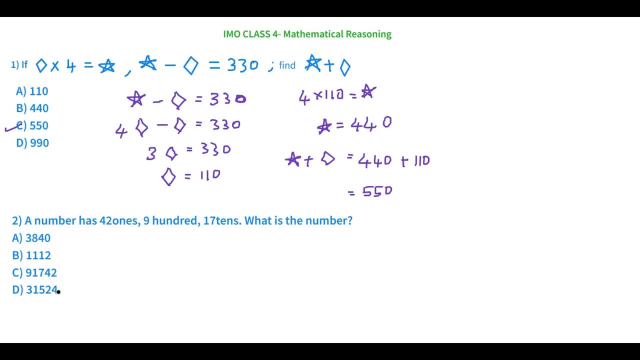 Option D is 524.. So let us see which is the right answer. So a number has 42 ones. So 42 ones means 42 times 1., So which is 42. And 900.. 900 means 9 times 100, which is. 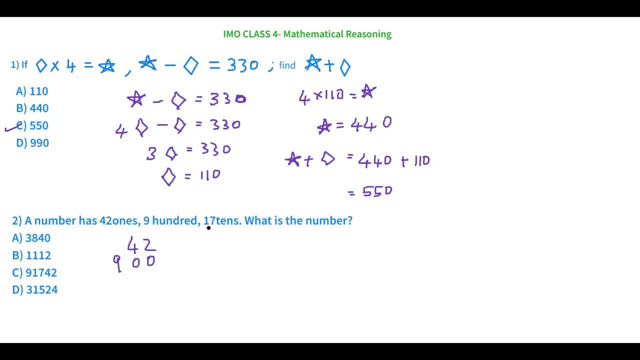 900.. And 17 tens. 17 tens means 17 times 10, which is 170.. So we have to add up all this. Let us see what do we get. We get a 2 here. 4 plus 7 is 11.. 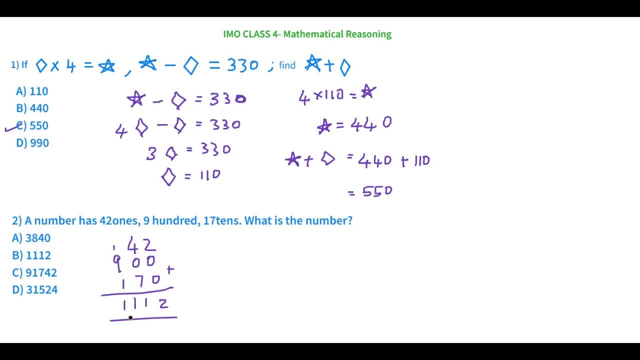 And then we have a 10 and then 11.. We got our answer as 1112.. So our final answer is 1112.. Isn't it very easy. We just need to find out 42 ones. We will multiply by ones. 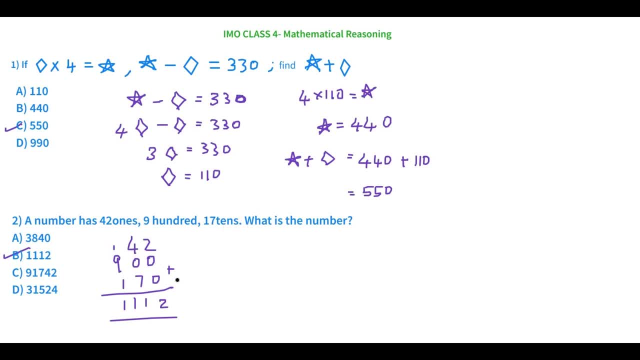 If it is 100, we will multiply by 100. And if it is tens, we will multiply by tens and then add up all these numbers And we get our final answer. And if you found this video interesting, do not forget to click on the subscribe button. 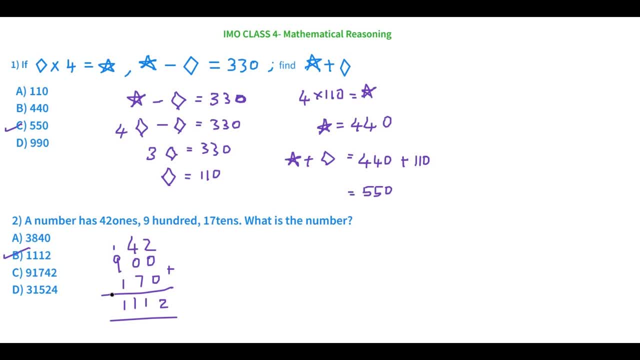 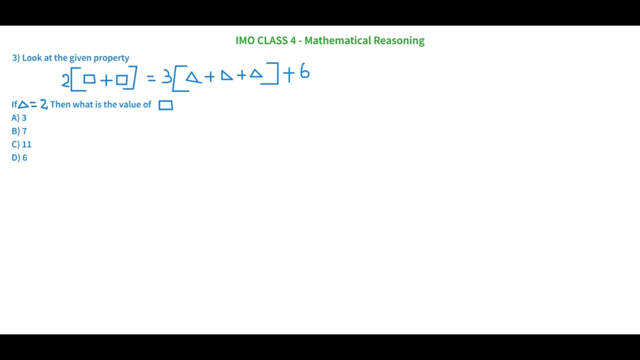 And do not forget to click on the bell icon so that you get a regular updates of all my videos And if you liked the video, click on the like button. Now let us see the third question for today, which is look at this given property. So 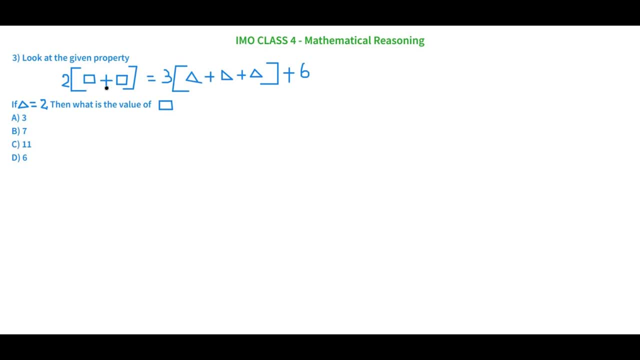 let us see what is given 2 times. there are 2 rectangles, That is, rectangle plus rectangle. 2 times rectangle plus rectangle equals 3 times triangle plus triangle plus triangle plus 6.. So this is the property given to us: 2 times rectangle plus rectangle equals 3 times triangle plus triangle plus triangle. 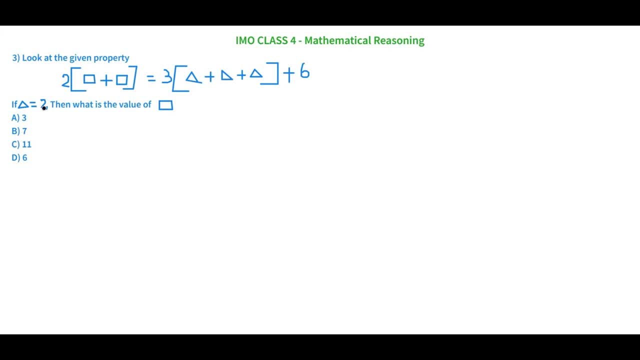 plus 6.. And then if triangle equals 2, so the value of triangle is given to us, Then find the value of a rectangle. So first let us take the left hand side, right pause. Now let us take the right hand side. that is 3 triangle plus triangle plus triangle plus 6.. So in place. 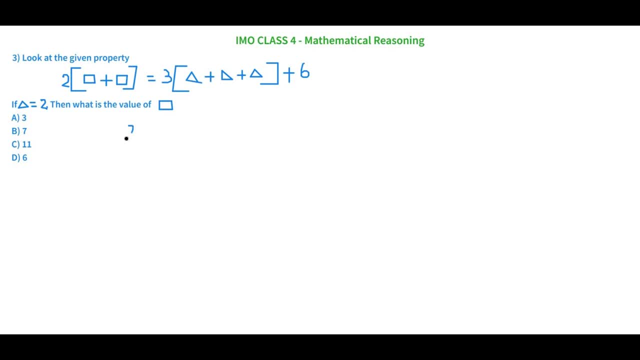 of triangle, I am gonna directly going to substitute it as 2.. So 3 times 2 plus 2 plus 2, and then there is a plus 6 outside. So let us find the value of the left hand side. 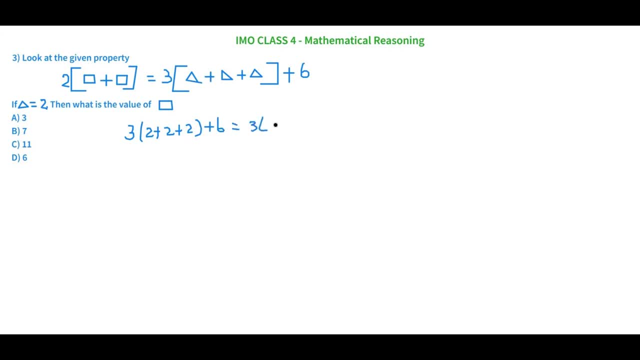 So what do we get? 3 times 2 plus 2 plus 2 is 6 plus 6.. So 3 times 6 is 18.. 18 plus 6.. So 18 plus 6 played out against our combination of 2 plus 2 plus 6 plus 6.. And we would now: 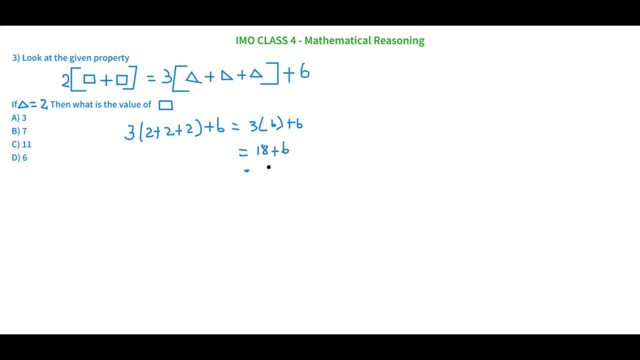 6.. So 18 plus 6 is equal to 24.. So we have got the value of the right hand side. Now let us see the left hand side. What is given in our left hand side? 2 times of 2 rectangles There are. 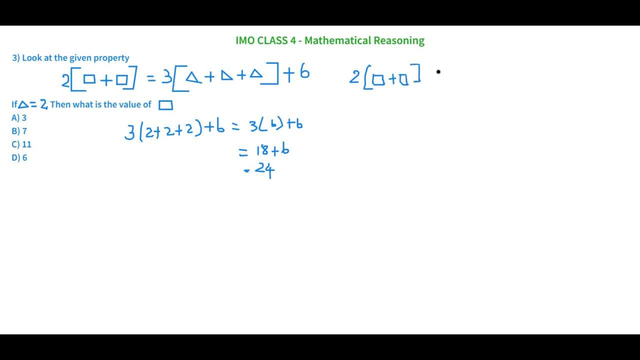 2 or 1 rectangle plus another rectangle equals what is the right hand side value we have got. We have got it as 24.. So now 2 times 2 rectangles equals 24.. So then 1 rectangle plus another rectangle equals 24 divided by 2.. So this 2- I am taking it this side, So it has become division. 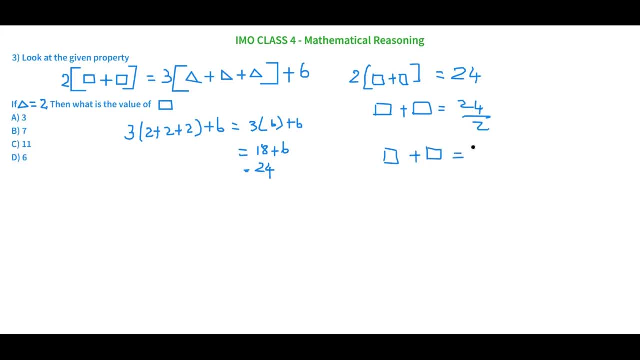 So now, a rectangle plus another rectangle equals 12.. So the 2 rectangles together makes 12.. So what is the value of 1 rectangle? 1 rectangle equals 6.. Isn't it easy? So do we have that option? Yes, we have an option here, So our correct answer is 6.. Isn't it pretty easy? 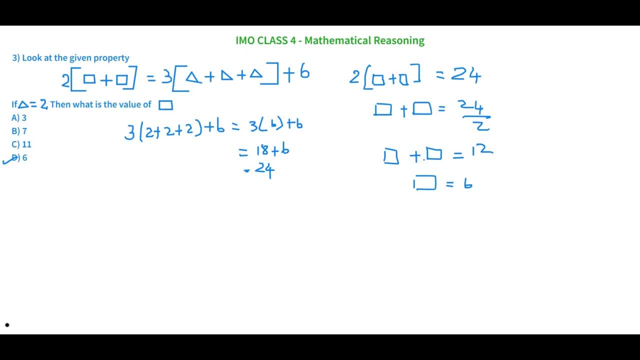 If you found this video interesting and easy, then please like, share and subscribe to our channel. Thank you. Easy for you to understand. Do not forget to click on the subscribe button and hit the bell icon so that you get a regular updates of all my videos. And if you like the video, do not forget. 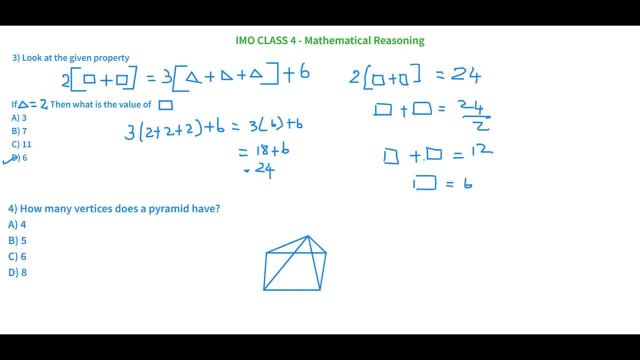 to click on the like button. Now let us see the fourth question for today. So the question is: how many vertices does a pyramid have? And we have the option of 4,, 5,, 6 and 8.. So let us So now let us see: how many vertices does this pyramid have? 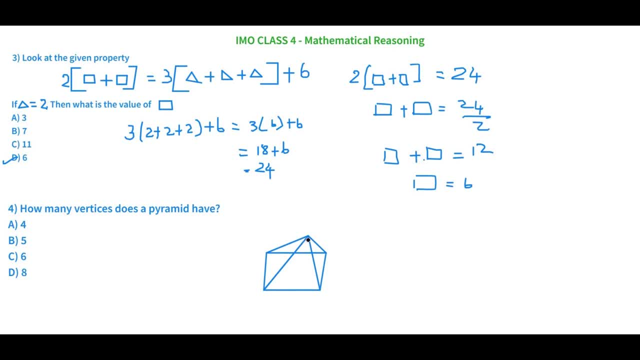 Vertices is nothing, but where the 2 straight lines meet is called as a vertices. So let us see what is. how many vertices does the pyramid have? So the points where it meet, this is 1 vertex 1, 2, 3,, 4, 5.. So a pyramid has how many vertices? A pyramid has 5 vertices, Isn't it easy? 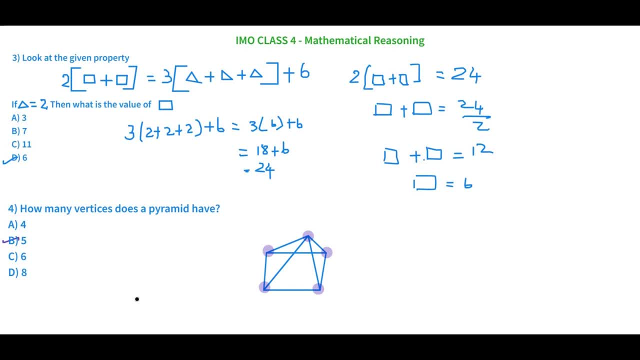 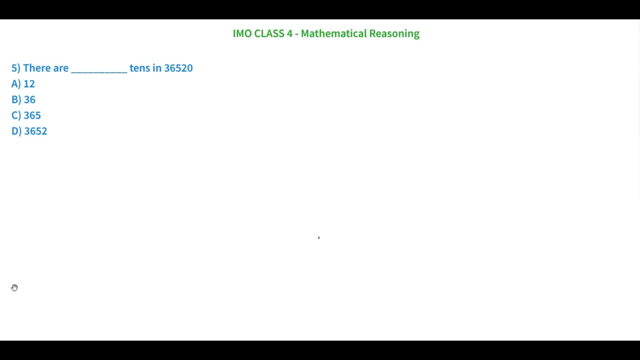 So always remember, vertices are the points where 2 or 3 lines meet. that is that is called as a vertices. Now let us see the fifth question for today. There are dash 10s in 36,520.. So we have to see how many 10s are there. A pretty easy trick is when we have a number like 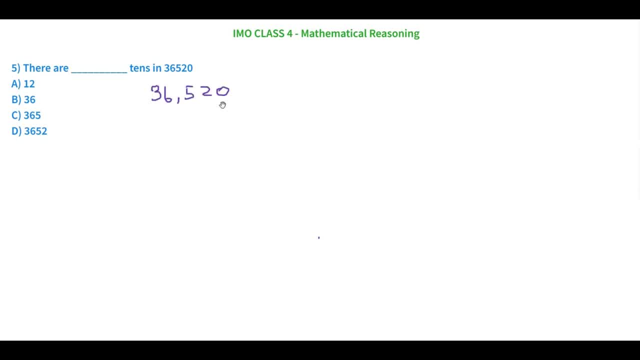 36,520.. So we have a number like this. Then what is the question asked? We have to know how many 10s are there. So we will start from the 10s place, that is, this 2 is in our 10s place- and write the all the numbers. 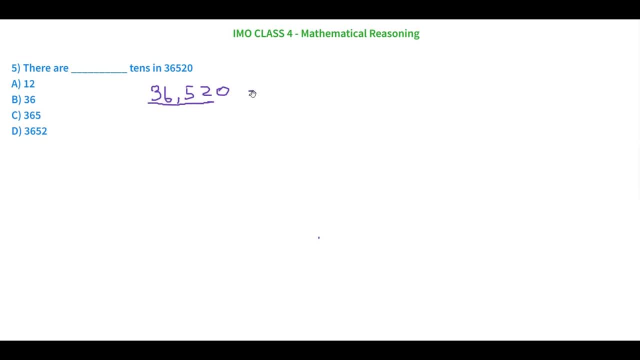 behind. So what is our answer? How many 10s are here in this? We have 3,652 10s. We can write like this: Since 10s has been asked, we will write it from the 10s place. So for this question, the 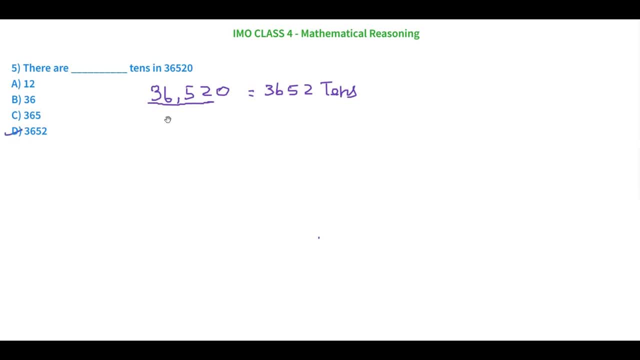 answer is 3,652.. For example, if they are asking you how many thousands are there, So 36,452.. How many thousands are there? Usually we write it as there are 6,000s. No, that is wrong, So you. 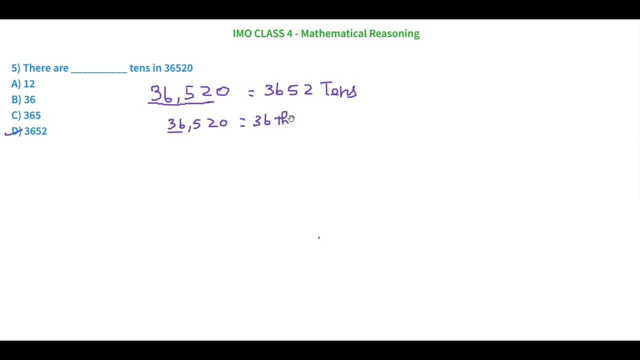 take it from behind So you can write it, as there are 36,000s. So it is a very easy thing. We will start from the place which has been asked. For example, if it is asked like how many hundreds are here, How many hundreds are there in this number? So it is pretty easy, From the hundreds. 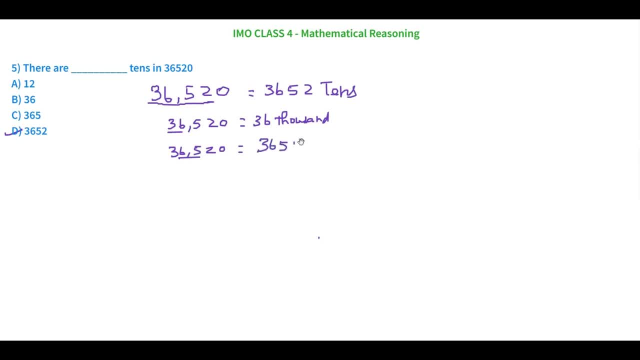 place you will write everything. So we have 365 hundreds, Isn't it easy? However, this type of question is asked from the place which has been asked. you will write all the numbers. So you will write the behind numbers, Right, So isn't it very easy? This is a small. 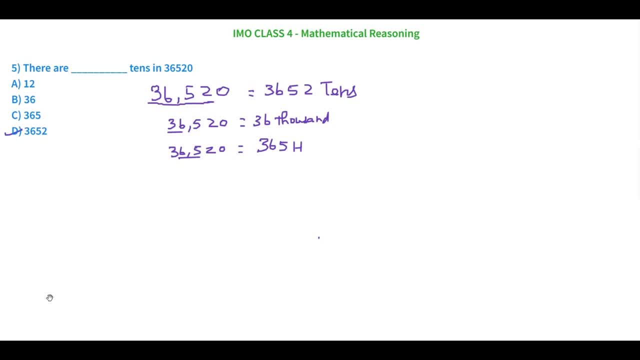 trick which you can apply for your exams. And if you found this video interesting and if you are able to understand it clearly, click on the subscribe button and hit the bell icon so that you get a regular updates of all my video. And if you like the video, do not forget to click on the. 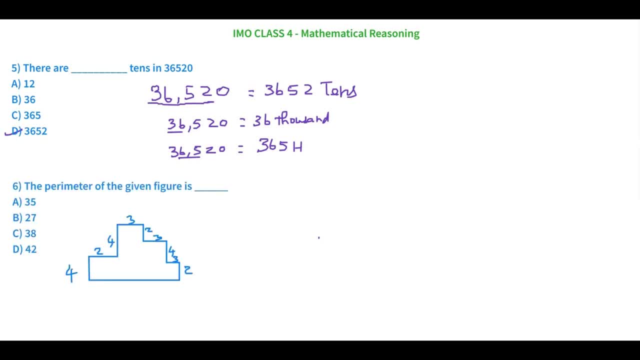 like button. So now let's see the sixth question for today. The perimeter of the given figure is blank, So we have to find the perimeter of this figure. The options given to us are 35,, 27,, 38, 42.. So we. 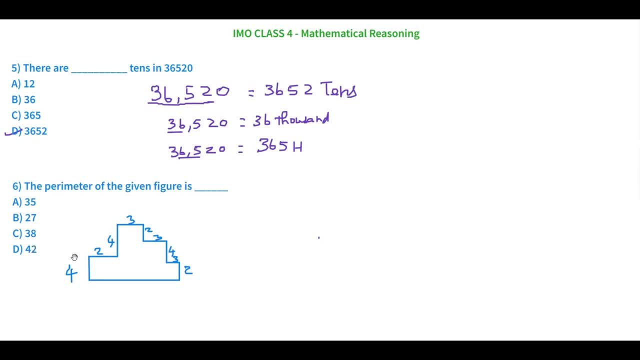 have to find the perimeter. So what is the perimeter? Perimeter is nothing but the outer sides. We have to add up the sides, Right? So how many of our sides are there? It is very easy to find a perimeter: We just need to add the sides. But all the sides are given. What about the? 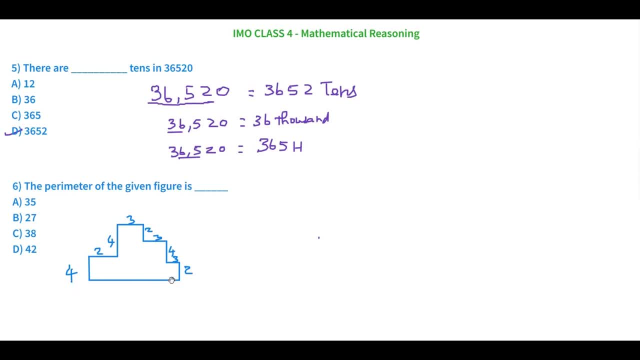 side. This bottom length is not given. How will we find that We can add up the remaining sides? but what about the bottom side which is not given? First we have to find the bottom side. Now we don't know the bottom length. that is the horizontal line. So to find that it is pretty easy, Do not? 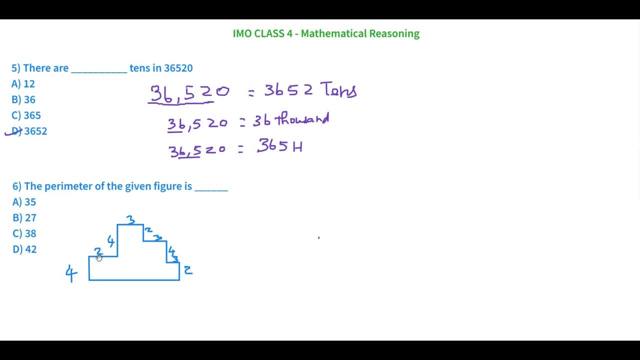 get confused. It is very easy. You can see this horizontal line. There is a horizontal line here. till this it is 2.. So we have the length. till this it is 2.. And then, as you can see, there is another horizontal line of length, 3.. So, which is till this: 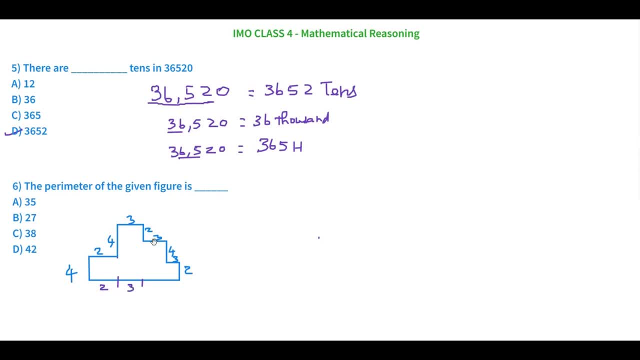 We have our length as 3.. Now again we have another horizontal line of length 3.. So that is till this. we have another horizontal line of length 3.. And then again another horizontal line of length 3.. So, as you could see, this whole length is here given in this part. So we have a 2,, 3,, 3, and then 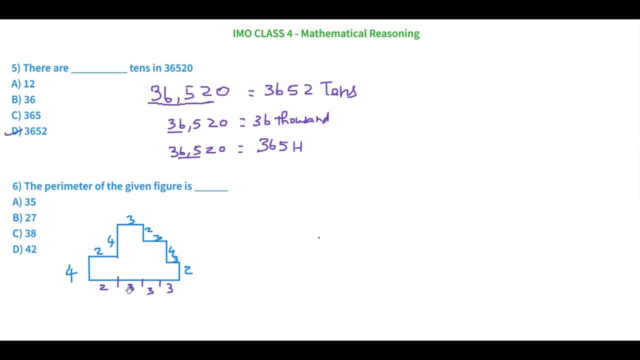 again a 3.. So what is the total length of this? 3 plus 3 is 6.. 6 plus 3 is 9.. 9 plus 3 is 11.. So now we have found the total length of this length.